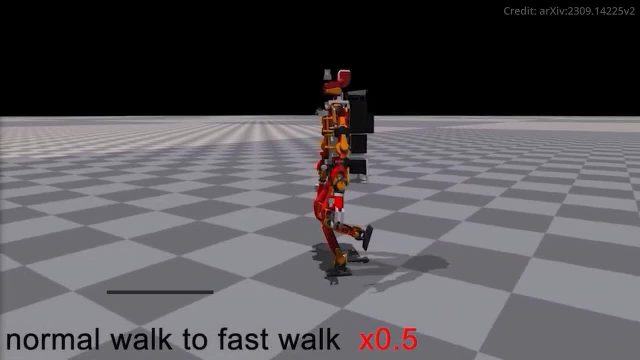 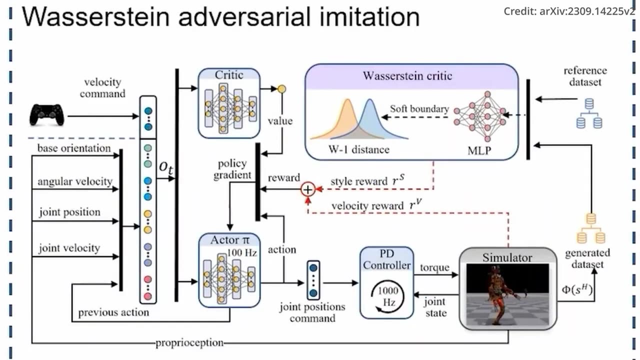 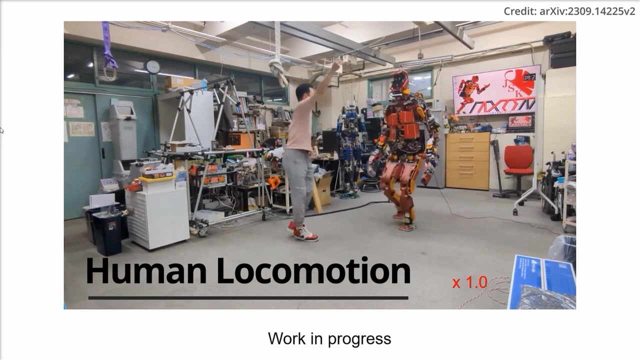 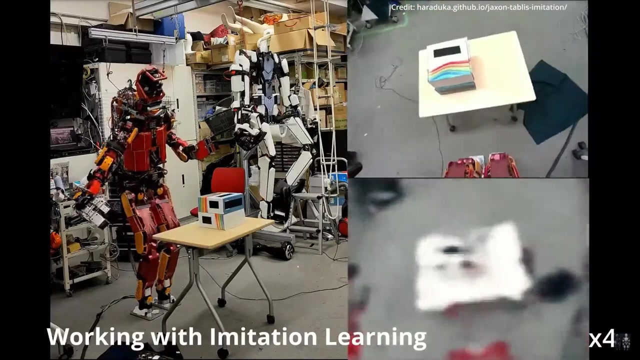 ETH Zurich. In this groundbreaking development known as Human Mimic, these researchers have introduced the Wasserstein adversarial imitation learning system as a breakthrough leap towards enabling humanoid robots to mirror human locomotion with an unprecedented level of fluidity and precision. See: human motion is a complex combination of muscle activations. 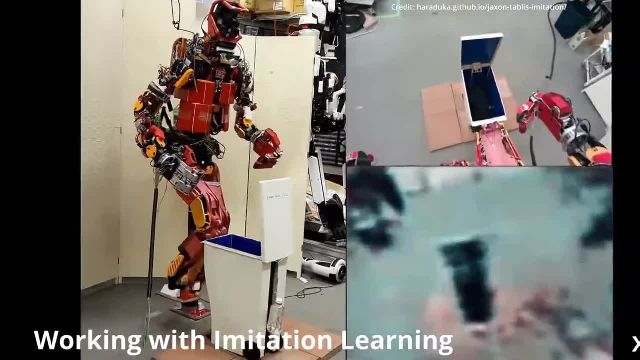 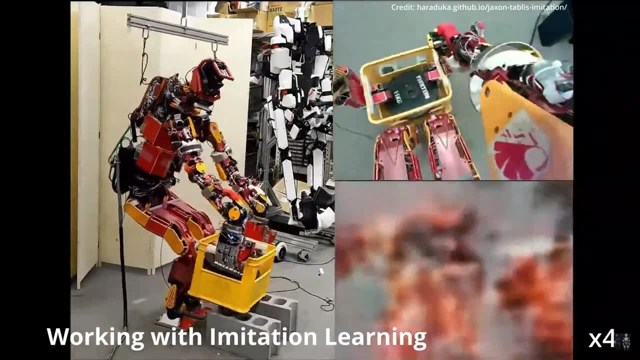 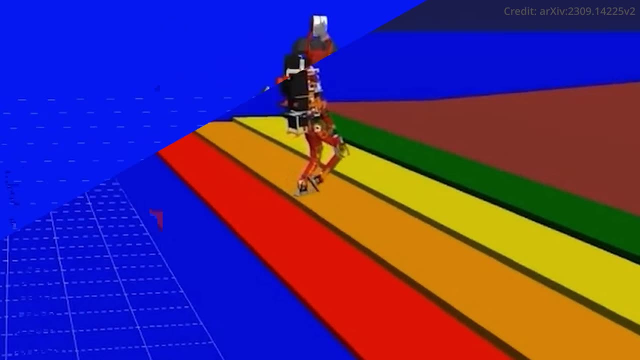 joint movement and balance control. but given the control complexity and the nuanced motion design required to navigate our physical world, transferring this intricate orchestration of locomotion and adaptive gait transitions to humanoid robots has always been a herald. The 800 people trained to master the WPTR-1 AI research have been evaluated in every. 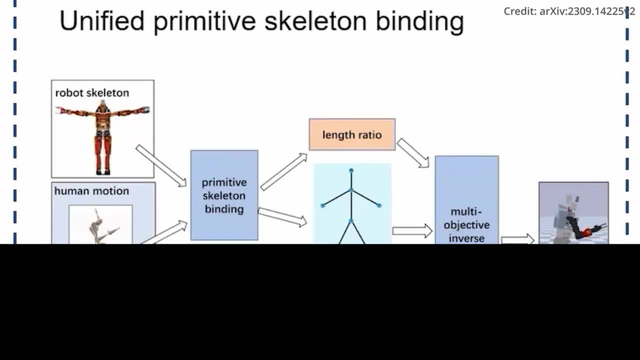 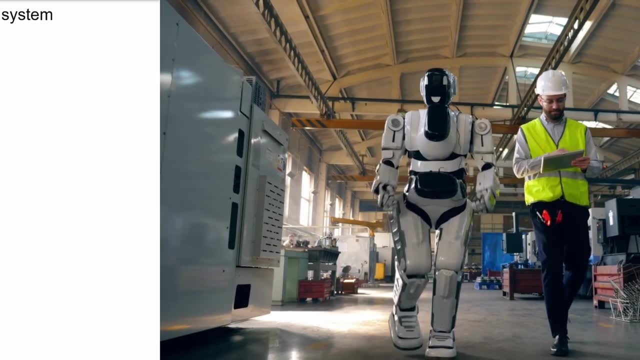 way. based on their expertise and effort Afterwards, the team of AI researchers have developed a new software that supports the WPTR-1 AI research with a new, improved além of the rota-skeleton-file that can help us control the scales on our bodies. 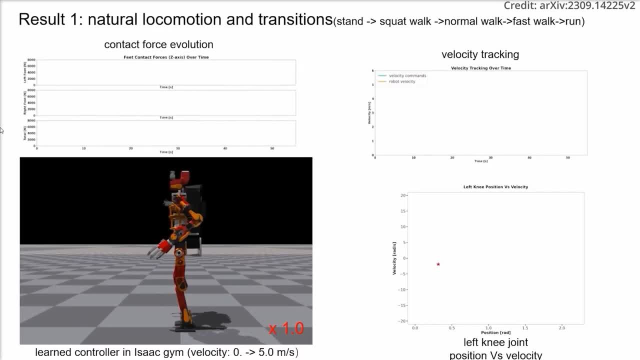 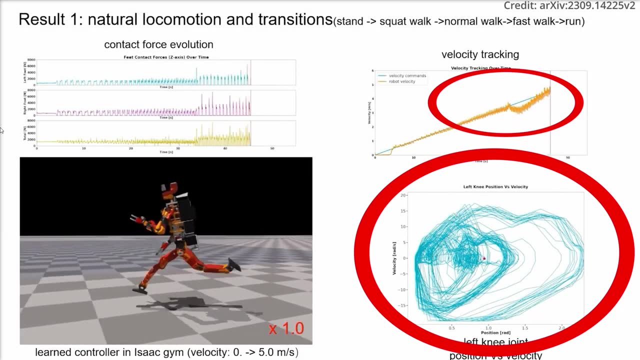 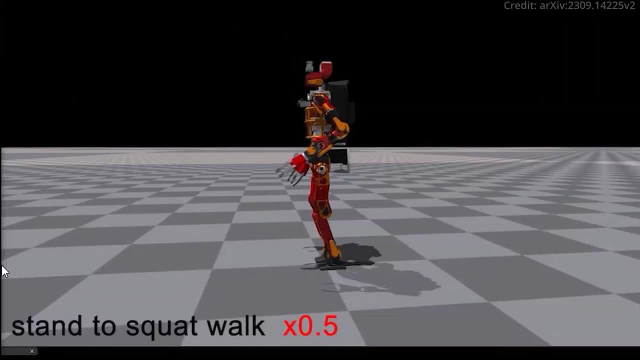 In addition, the team of AI researchers have installed a new, unique primitive-skeleton-motion retargeting approach to finally bridge the divides of morphological, and the forthcoming control policy is nothing short of revolutionary, demonstrating a spectrum of locomotion patterns including standing, push, recovery, squat, walking. 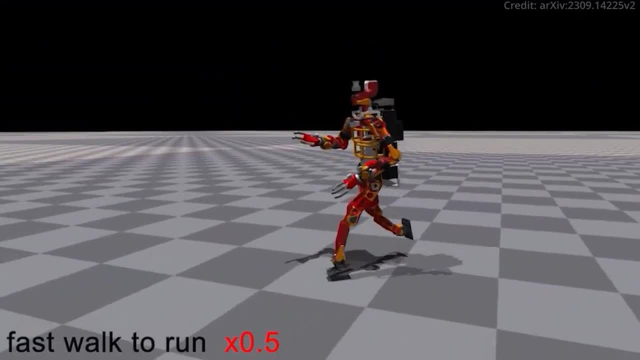 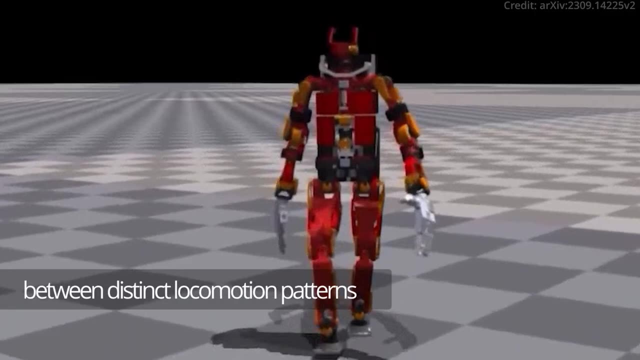 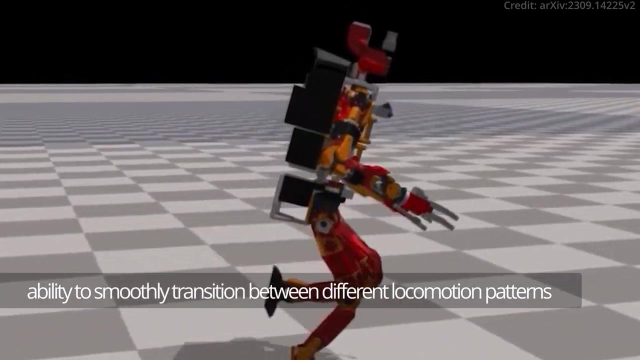 human-like straight leg walking and dynamic running. Furthermore, their humanoid robot named Jackson can both execute and naturally transition between distinct locomotion patterns, as the desired speed changes This ability to smoothly transition between different locomotion patterns, particularly in the absence of transition motions in the demonstration dataset. 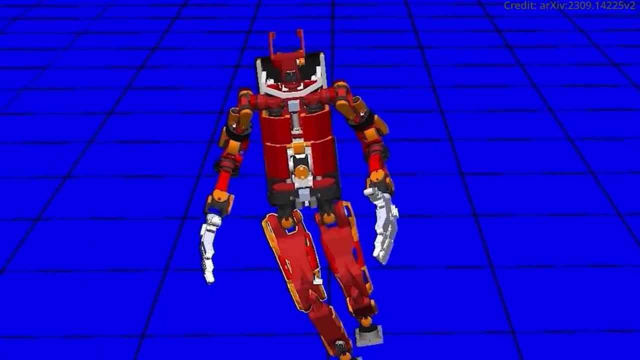 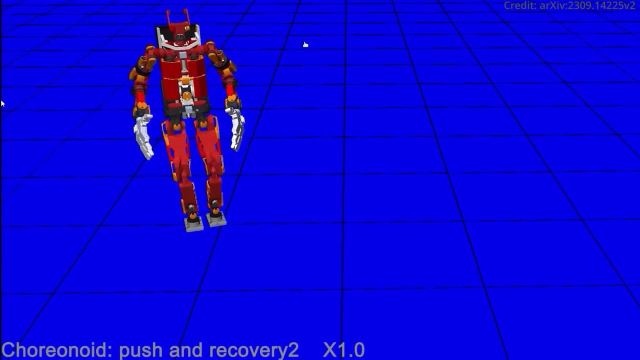 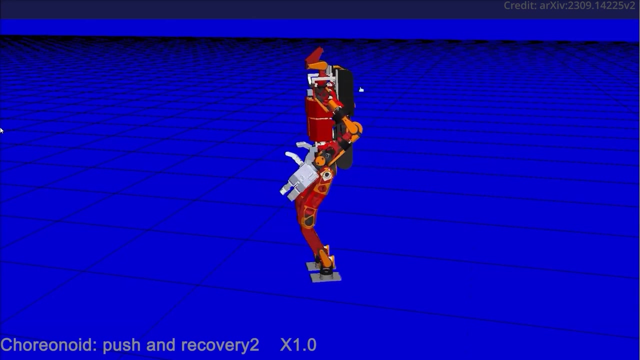 is a marvel in robotic locomotion, But navigating through the complexities of robot locomotion with deep reinforcement learning has brought researchers face-to-face with both opportunities and obstacles. Despite deep reinforcement learning's ability to develop sophisticated movement in robots ranging from four-legged creatures to upright humanoids, 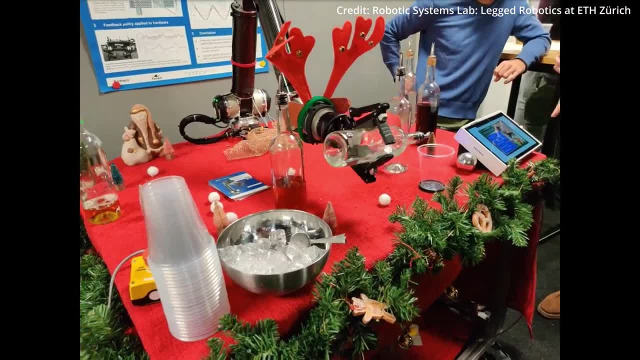 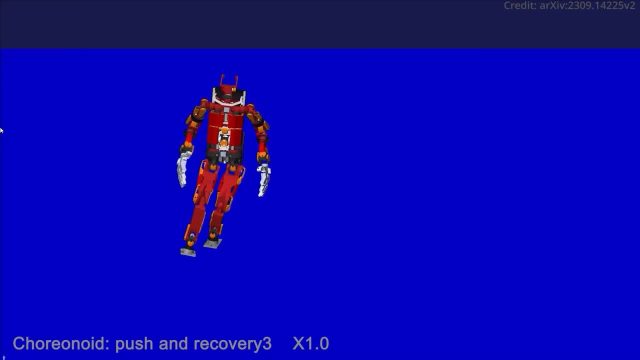 challenges like unnatural full-body behaviours and erratic arm movements have persisted. To mitigate these problems, the researchers melded an adversarial critic component with reinforcement learning, thus steering control policies towards behaviours that sync with a range of reference motions, Additionally by employing another discriminator. 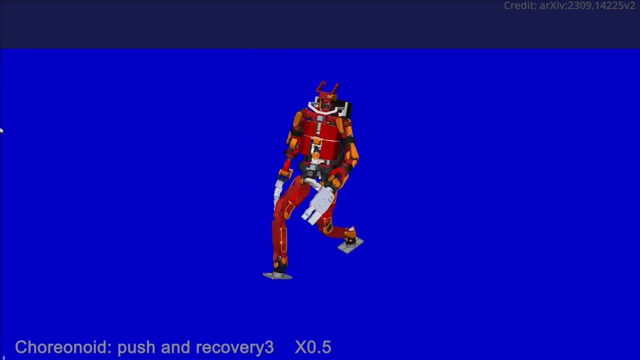 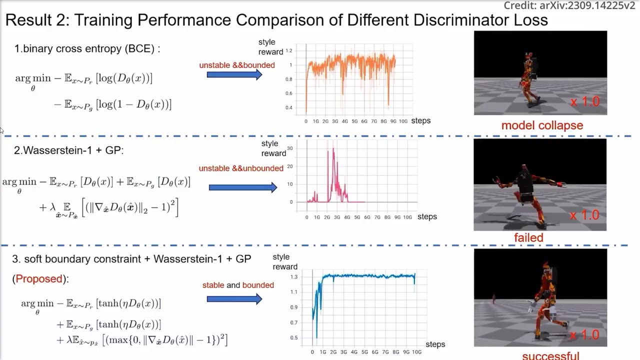 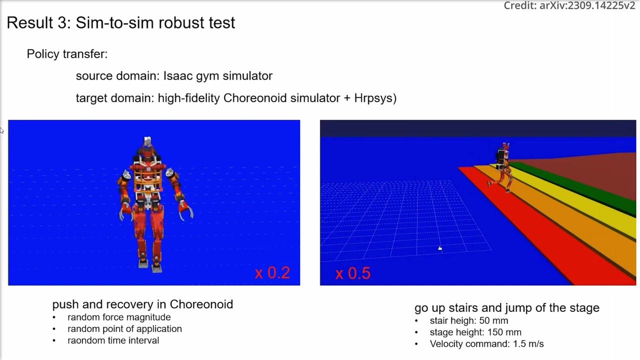 the adversarial motion prior incentivises the creation of motions that closely emulate human actions. But the journey wasn't without hurdles, because the discriminators trained with binary cross-entropy or least-square loss were often mired with unstable training and model collapse. In response to these setbacks, the researchers turned to integral probability metrics. 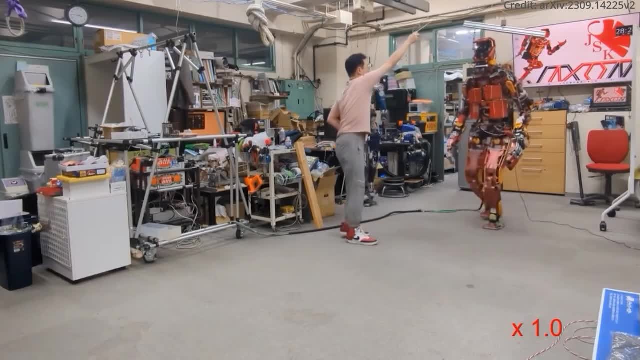 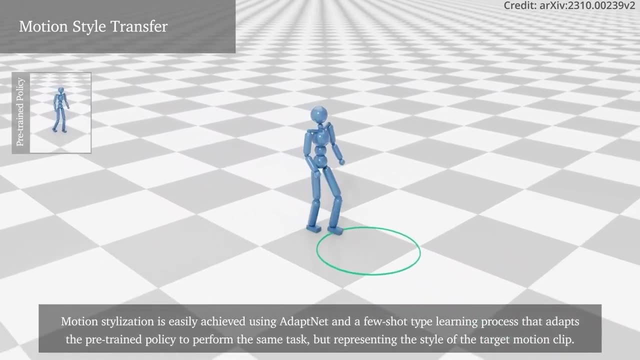 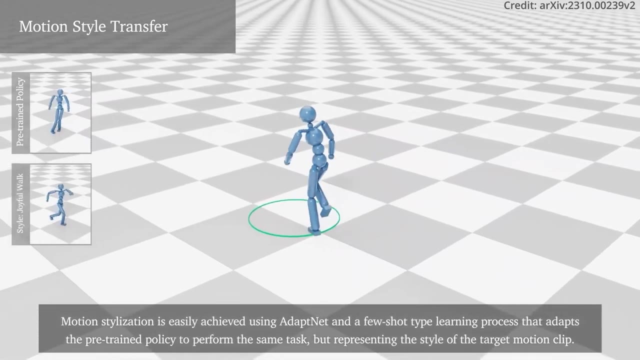 notably the Wasserstein distance, to stably and successfully navigate through these challenges. But, even more incredibly, yet another human locomotion. AI was recently unveiled as a groundbreaking approach to redefine physically-based character control, and the results have been truly astounding. Enter AdaptNet, an innovative character control technology. 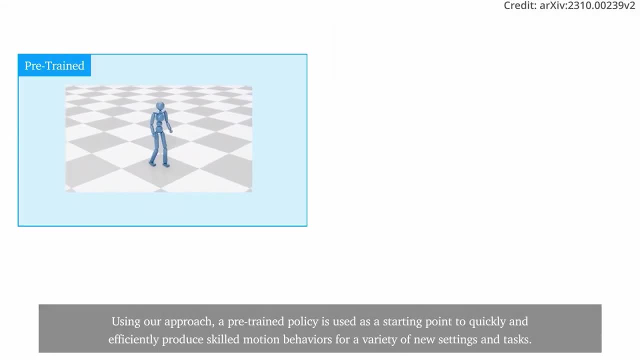 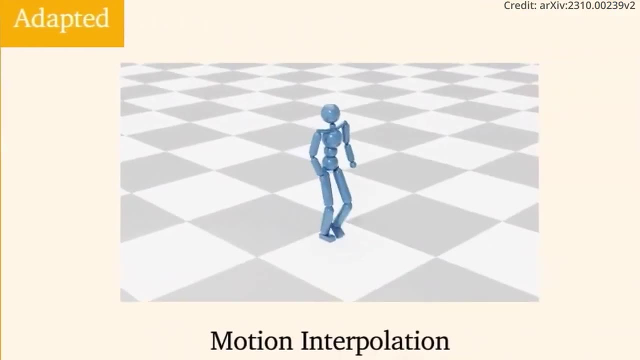 which has been used for a long time. AdaptNet is an innovative technology for quick policy adaptation to achieve a seamless and efficient mechanism for skilled motion behaviours across a myriad of settings and tasks, From motion stylisation, interpolation between styles, to morphological and environment adaptation. 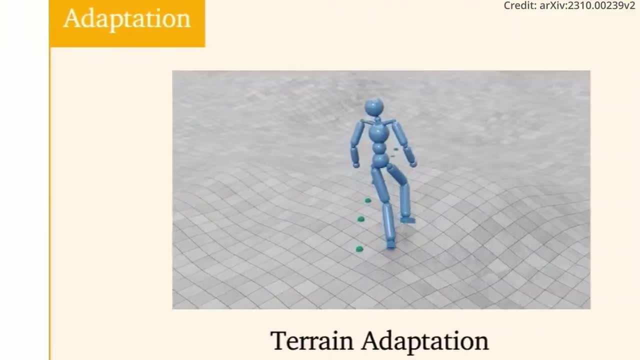 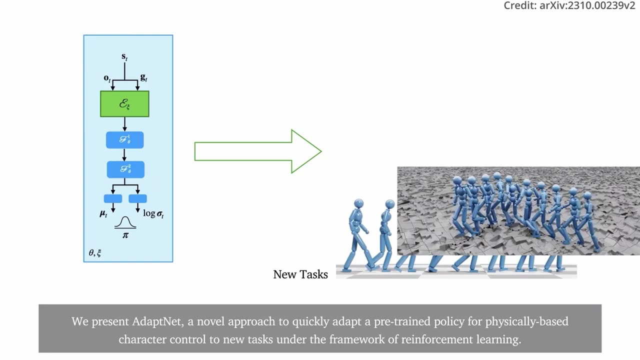 AdaptNet emerges as a versatile tool in the realm of AI and robotics. In fact, one of the stand-out features of AdaptNet is its capability to achieve motion stylisation using a few-shot type learning process. It adapts the pre-trained AI to the new technology. 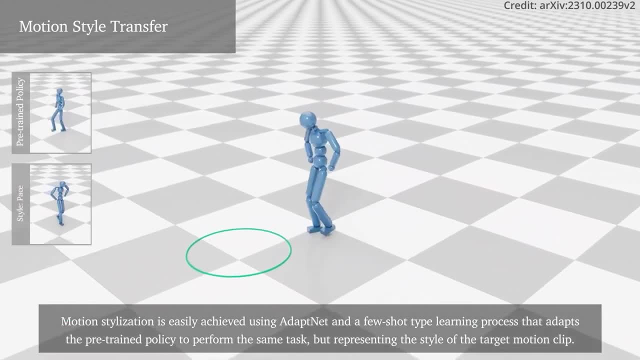 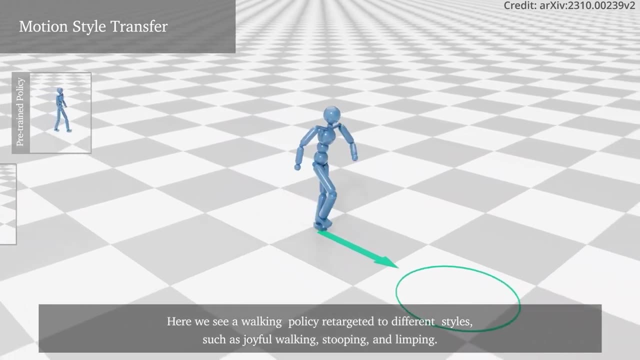 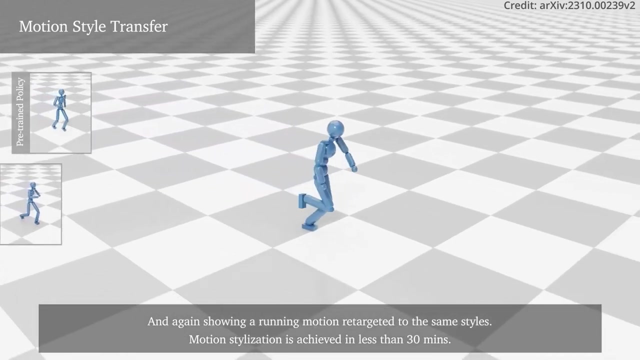 the pre-trained policy to perform identical tasks, but mirrors the style of the target motion clip, Whether it's a joyful walk, a stooping posture or a limping motion. AdaptNet retargets walking and running policies to different styles, achieving motion stylisation in under 30 minutes. 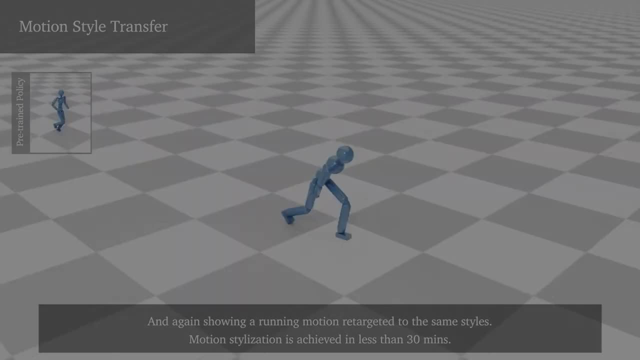 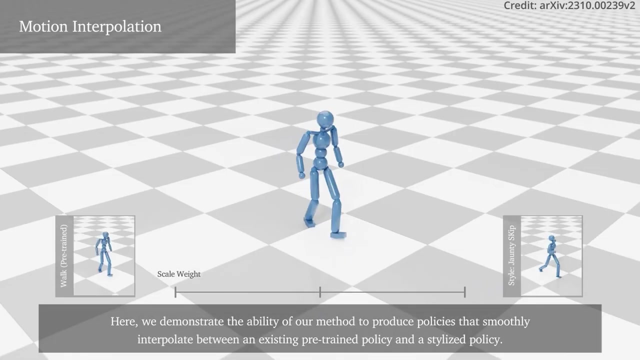 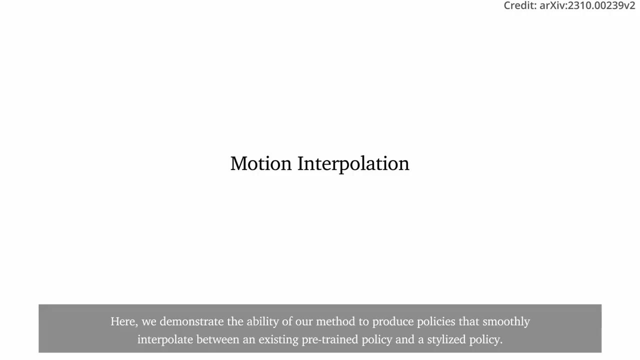 This rapid adaptation and stylisation of motions open up a world of possibilities in creating diverse and realistic AI characters in virtual environments. But AdaptNet doesn't just stop there. It also demonstrates a remarkable ability to produce policies that smoothly interpolate between an existing pre-trained policy and a stylised policy. 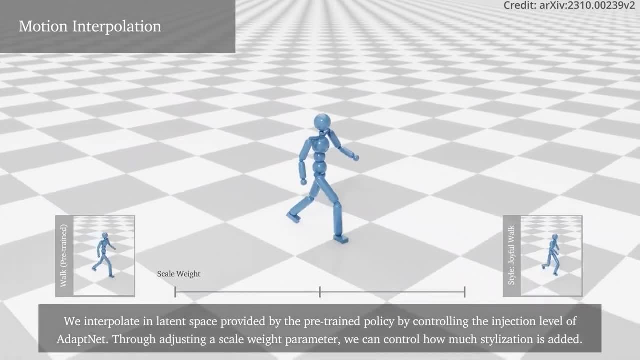 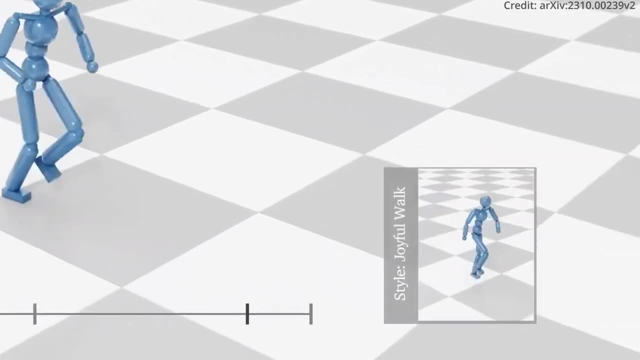 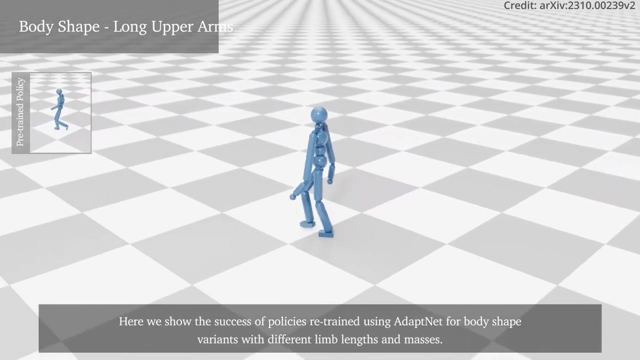 By controlling the injection level of AdaptNet and adjusting a scale weight parameter, users can control the degree of stylisation added, offering a nuanced and customisable approach to motion generation and control. In a world where one size doesn't fit all, AdaptNet shines by allowing policies. 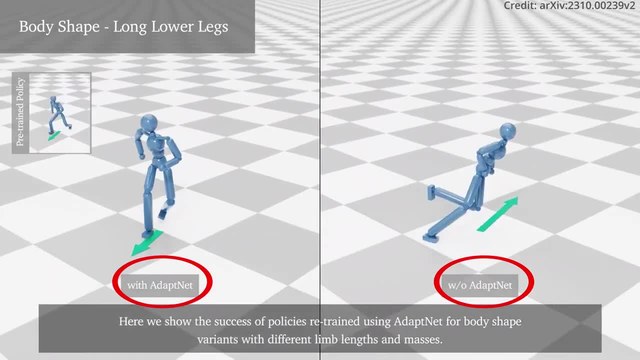 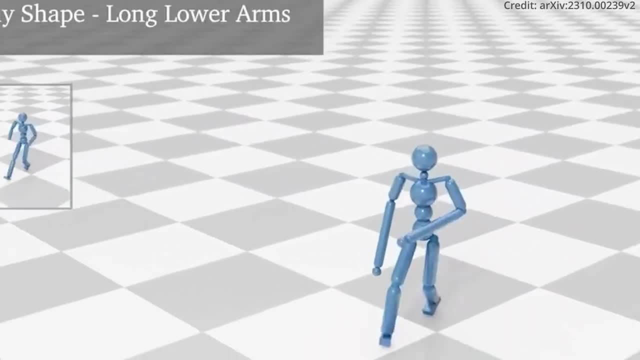 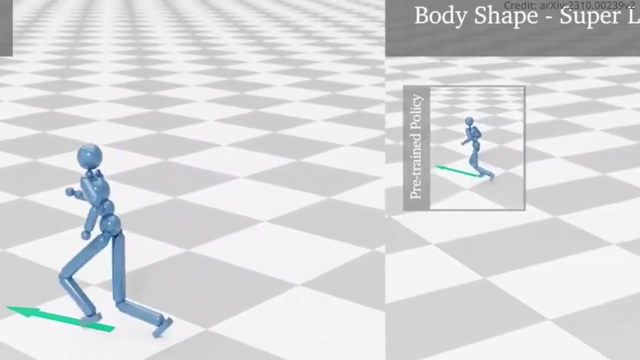 to be efficiently adapted to different character morphologies and dynamics too, From body shape variants, different limb lengths to varying masses. policies retrained using AdaptNet showcase success and effectiveness, ensuring that characters maintain balance and control even when morphological changes are introduced. 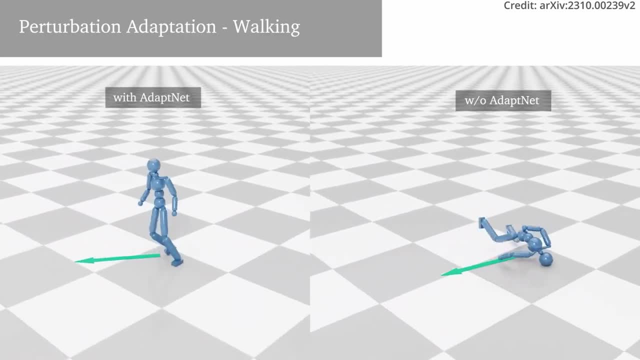 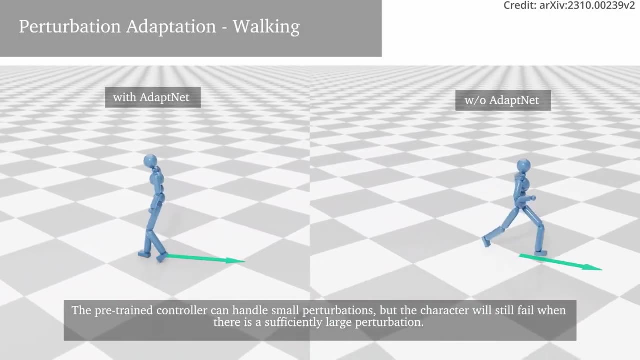 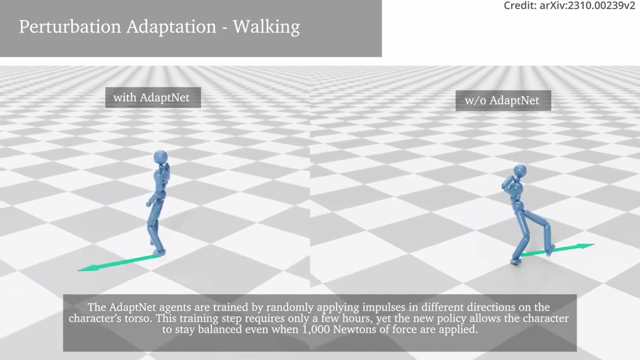 But AdaptNet goes a step further by enhancing the robustness of walking and running controllers Through training that involves randomly applying impulses in different directions on the character's torso. the new policy allows the character to maintain balance even under substantial perturbations, ensuring stability and control. 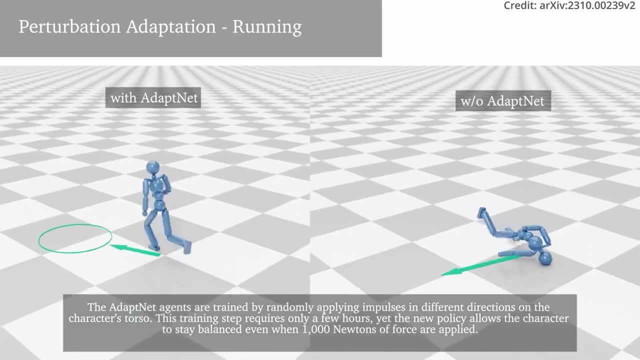 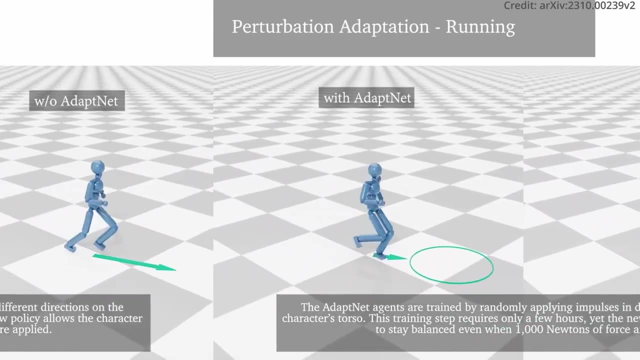 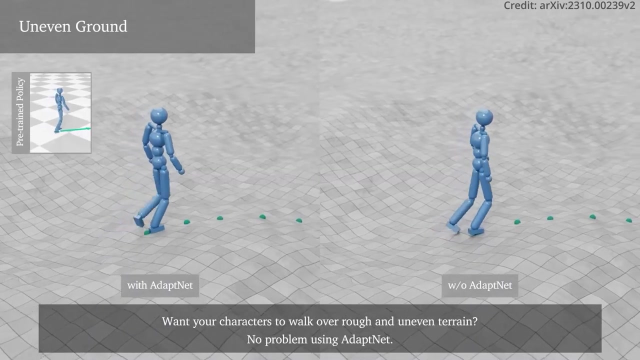 despite being put into purposefully difficult circumstances. Importantly, whether it's adapting to changes in friction coefficients or navigating through rough and uneven terrains. AdaptNet fine-tunes control policies to accommodate environmental changes By introducing a height map as an additional control input. 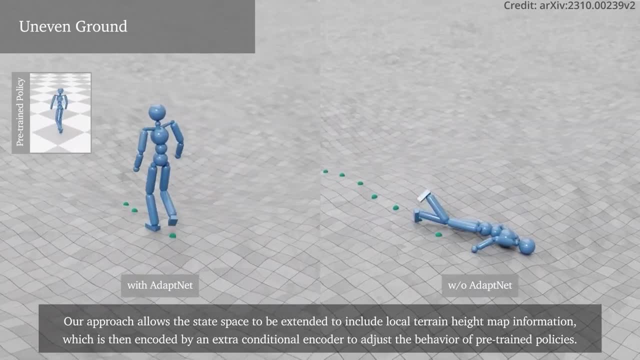 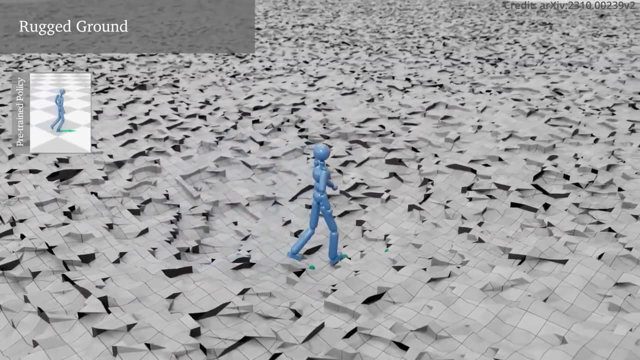 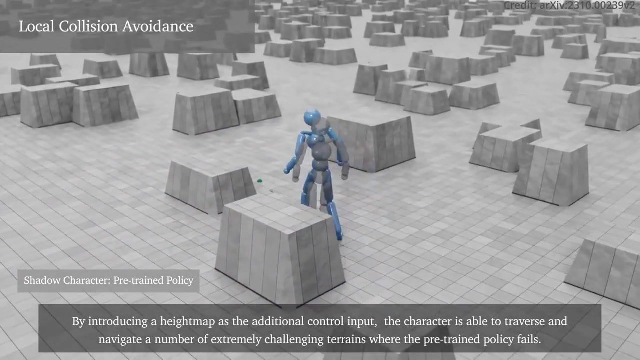 characters can traverse and navigate through extremely challenging terrains where pre-trained policies might fail, showcasing a remarkable adaptability to environmental variables. Furthermore, AdaptNet also extends its capabilities to local planning and obstacle avoidance, starting from a pre-trained policy without collision avoidance. 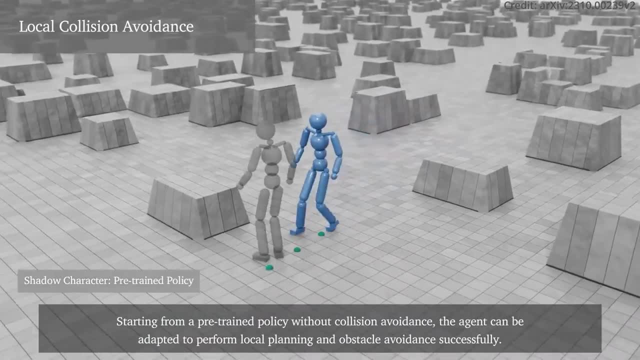 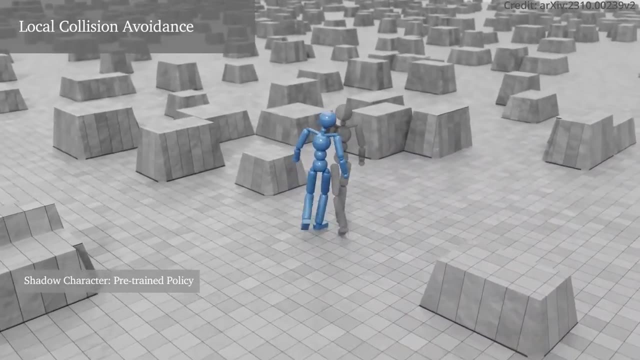 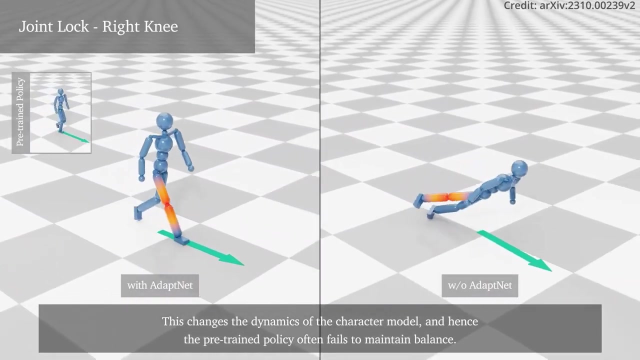 The agent can be adapted to perform local planning and obstacle avoidance successfully, showcasing a versatile application in real-world scenarios where obstacle navigation is crucial, Striking a balance between avoiding overfitting and ensuring the learning of stylized motions. AdaptNet demonstrates performance variations. 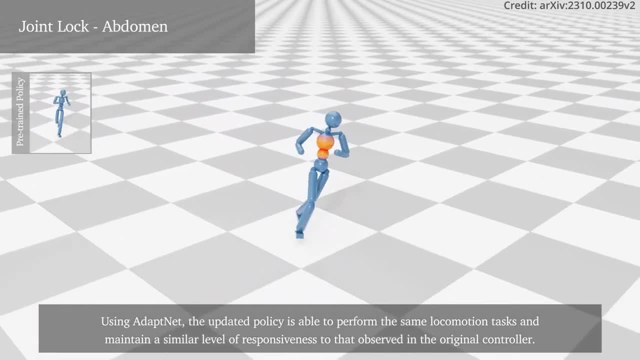 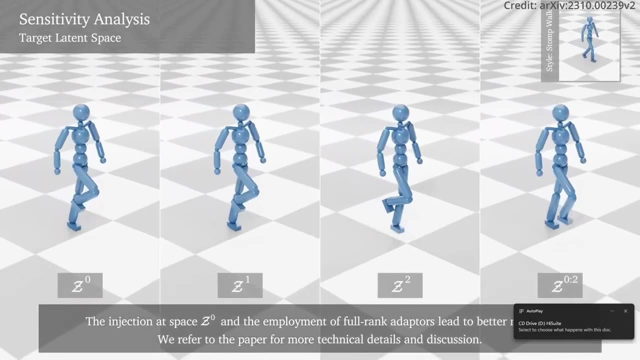 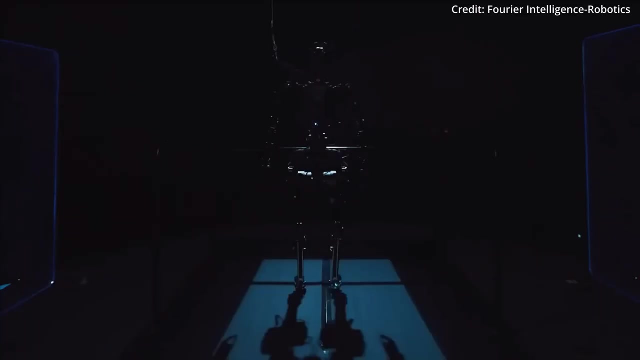 when different regularization is applied to the injected latents. This balance ensures that, while regularization is not always necessary, its application is crucial in certain tasks to prevent overfitting and ensure the successful learning of stylized motions In the near future. the rapid advancements of the 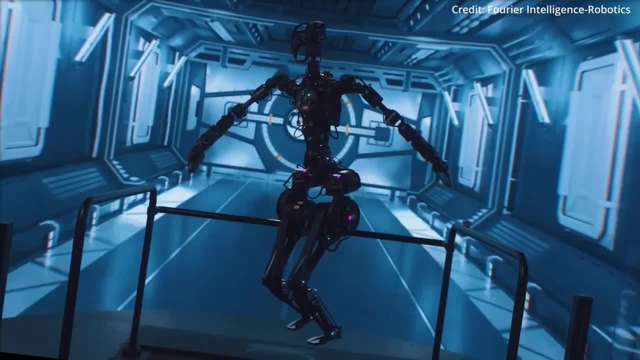 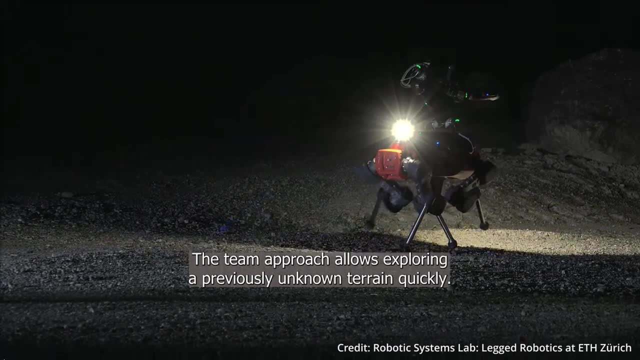 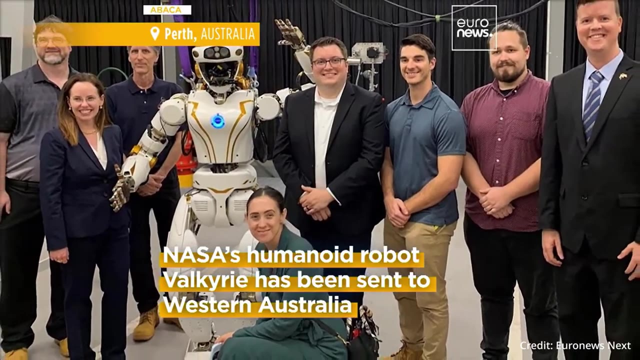 Wasserstein, Adversarial Imitation Learning System and AdaptNet will enable next-level teleoperation applications via robotics, particularly in executing tasks in dangerous or remote environments. Visualize teleoperated humanoid robots seamlessly executing complex, delicate tasks in hazardous environments like nuclear cleanup sites. 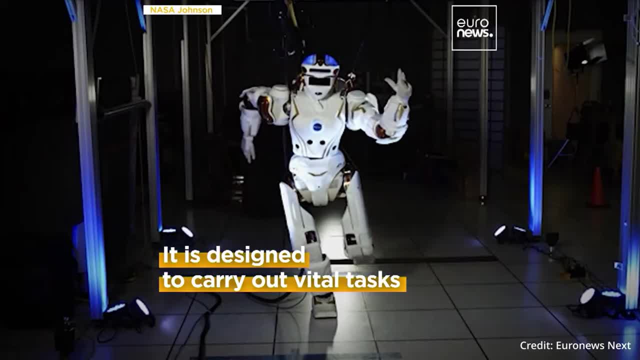 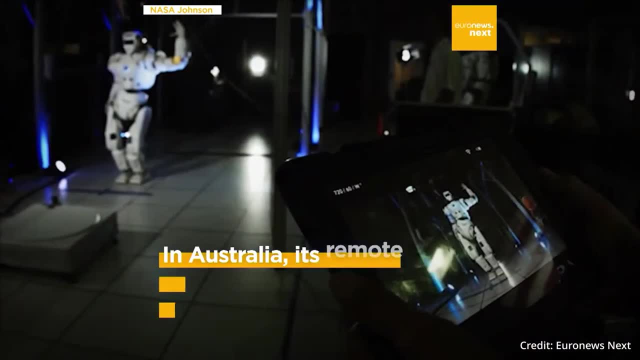 or extraterrestrial terrains where the conditions are too perilous or uncharted for humans to navigate safely. Such humanoid robots, armed with the ability to mirror precise human locomotion, could be manipulated from afar, ensuring human safety while marrying AI-driven human dexterity.